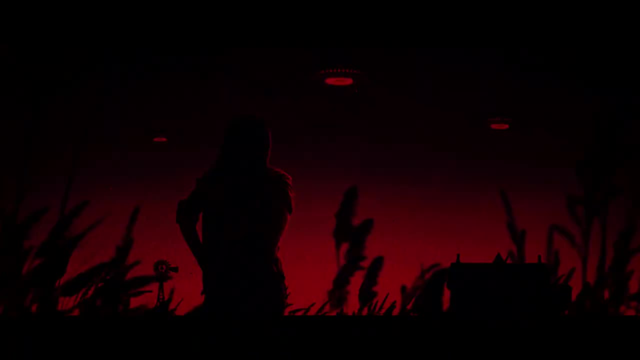 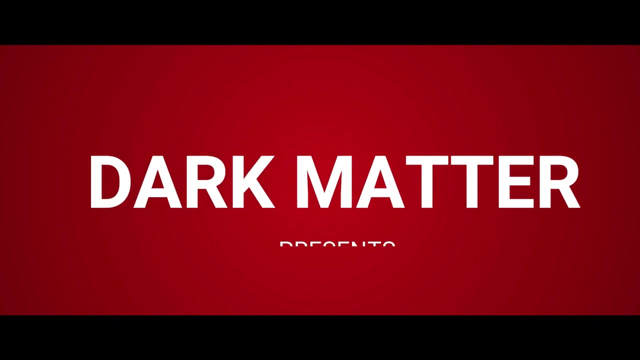 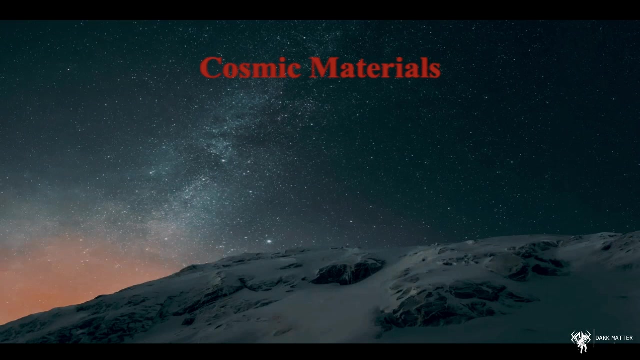 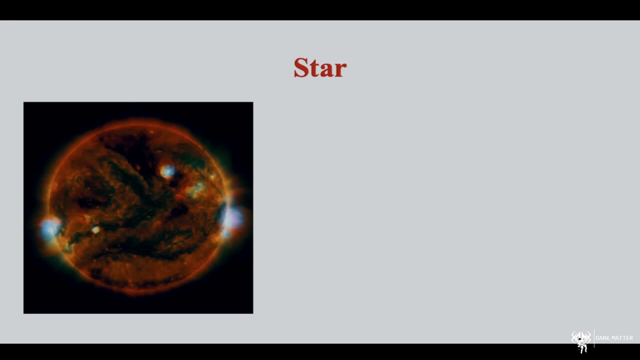 So in this lesson we will mainly study the cosmic materials or the celestial materials like stars, planets, satellites, galaxies, asteroids, comets, etc. So without wasting for the time, let us move into the study. So first we will study about a star. So a star is a luminous ball of gas, mostly hydrogen. 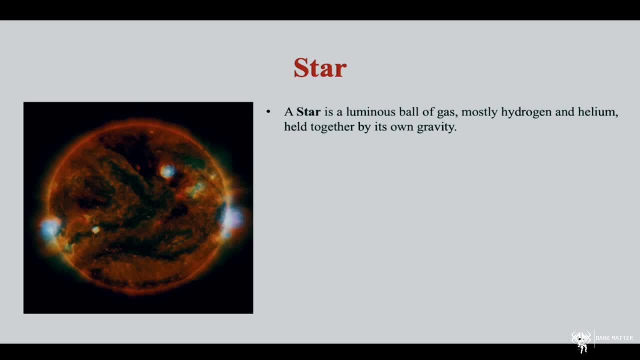 and helium held together by its own gravity. Nuclear fusion reactions in its core produce photons. Photons are basically the lights and heat. So, as we all know, all the stars have a luminosity, that is, they are luminous and they are very warm actually. So just to 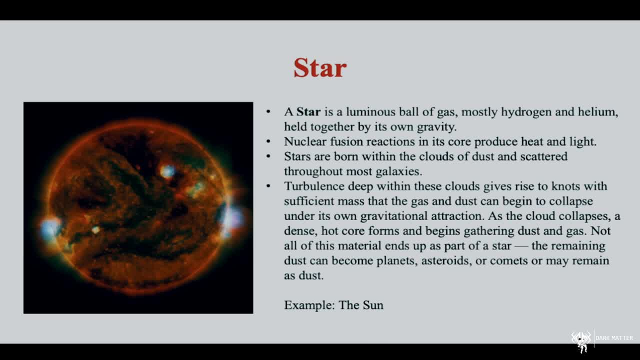 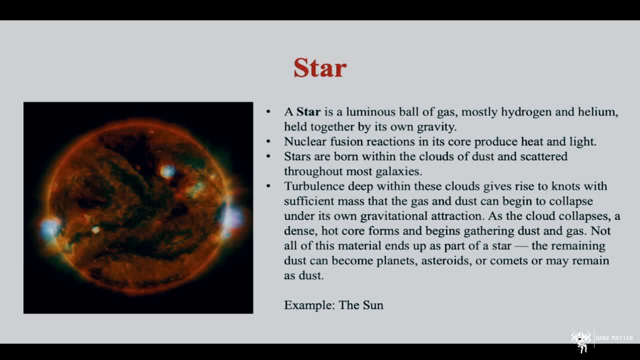 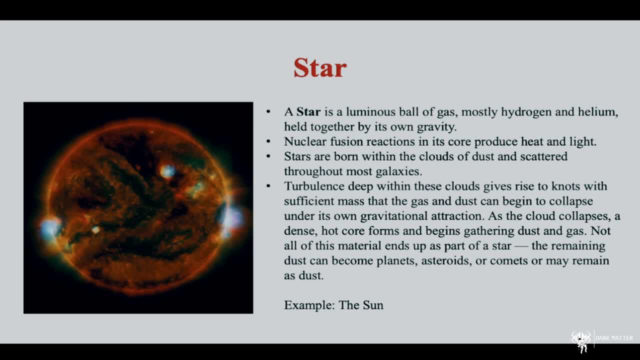 from the sun, you will actually burn into ashes, So you can imagine how warm, how hot actually a star is And, as I already told you, sun is a very good example of a star, basically, And there are other well-known stars as well, like Proxima, Centauri and also. 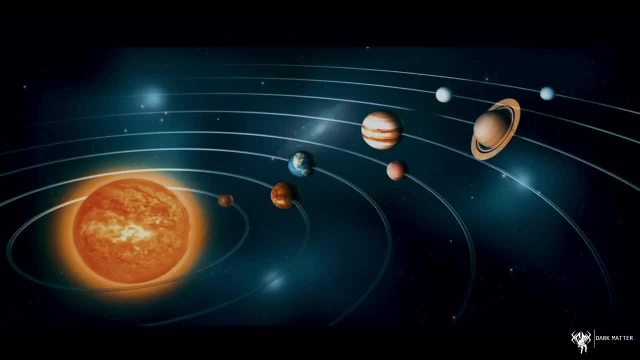 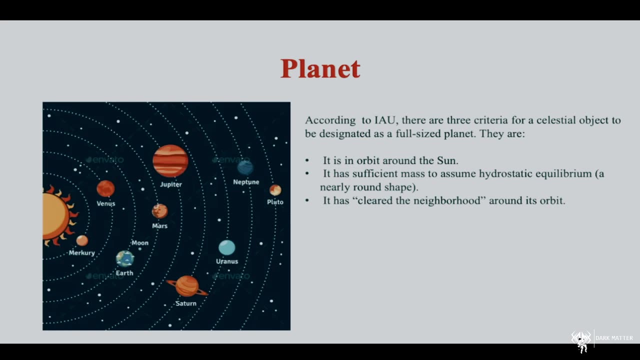 there are stars in our universe, Planet. Planet is a celestial object which is a big enough to have enough gravity to keep its spherical shape. That is, a planet is always spherical and planet orbits any star Like. a great example is our Earth, which is a planet, and it actually orbits around the 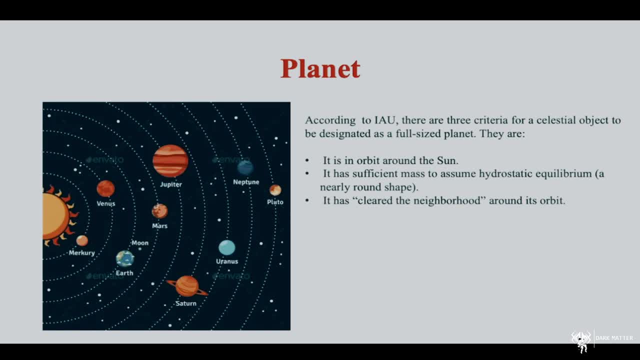 sun. So all the planets that actually orbit the sun are all together called the solar system. That also we know, And in this image you can actually see all the planets, although the spelling of Mercury is wrong here. I'm very sorry for that. actually, I've collected all these images from the Internet. 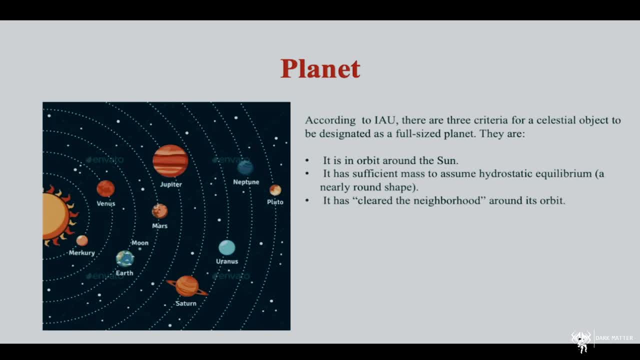 But somehow they wrote it wrong. And one note from this image is that Pluto is not considered as a planet in modern astrophysics because of its small size, So there are actually eight planets in our solar systems, Which we mean by eight? To measure those eight planets, we need a large number of planets in the solar system, But even if we do that, none of them seem to belong to Pluto. This is the only possible one. This world is a small, large planet, but one of it is small. The same thing is that Pluto is considered a planet in modern astrophysics because of its size. They are even larger than us, And so there are actually eight planets in our solar systems. 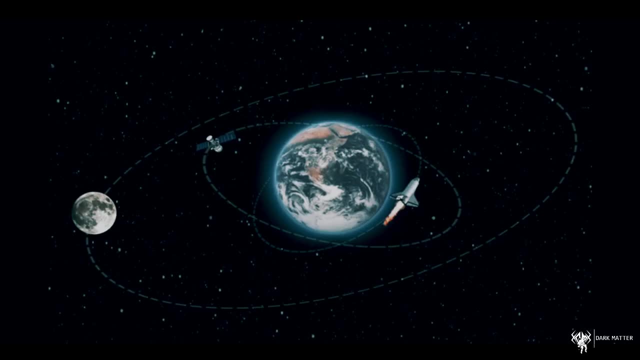 Satellite. a satellite is any celestial body in space that orbits around a planet. So satellites are of two types: natural satellites and artificial satellites. So as by their name you can say that natural satellites are those who are naturally present in the universe and artificial are those are made by human. 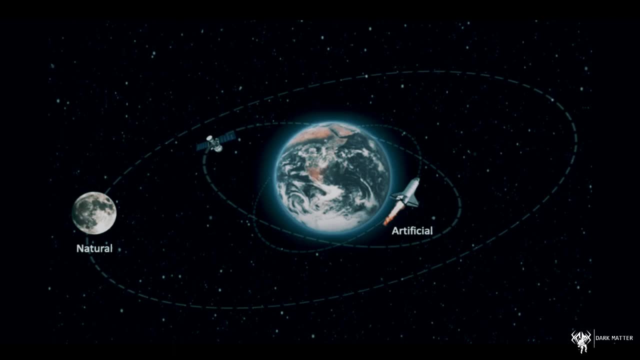 And human, like scientists actually send these artificial satellites from earth, definitely to study the universe or, at times, to use navigation, like the Google maps you use are basically GPS, the global positioning satellites used here. Those are also all those. all are actually controlled by these artificial satellites. 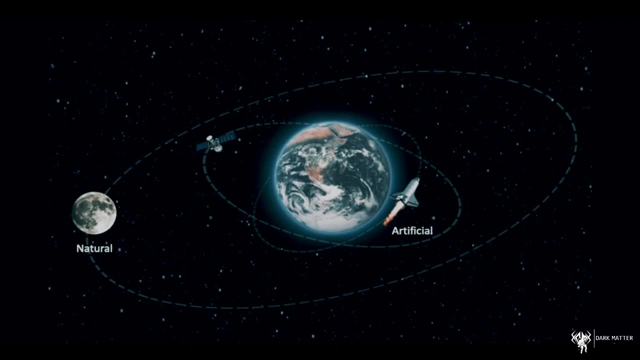 Those weather conditions, every type of things are actually monitored by a satellite. So satellites are of two types: moon, which are the natural satellites- moon is an example of natural satellites- and GPS, which is an example of an artificial satellite. So it's not necessary for all the planets to have a satellite, but few of the planets. 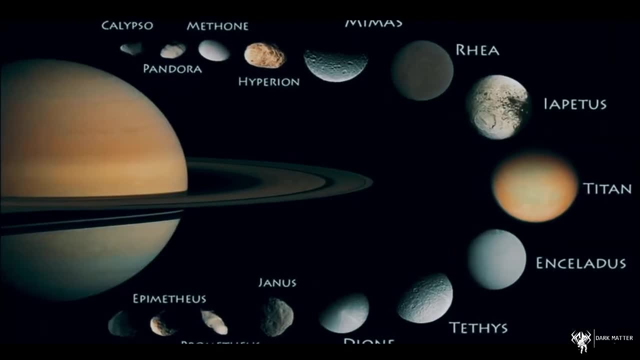 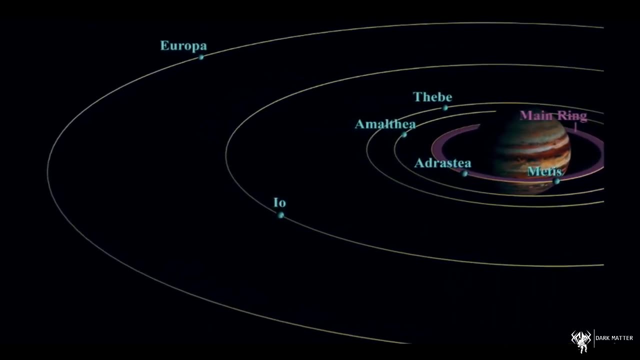 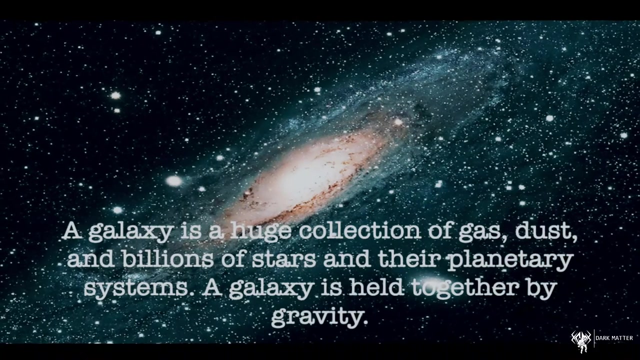 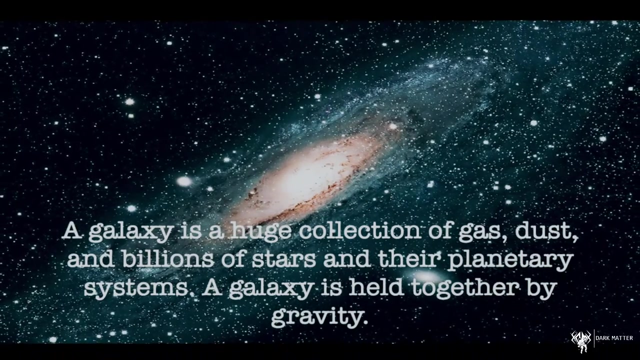 have more than one satellite. like Saturn, Jupiter, they have more than one satellite: A galaxy. A galaxy is a huge collection of gas, dust and billions of stars and their planetary systems, So actually you can imagine how big it actually is. It has billions of stars and their planetary systems as well.